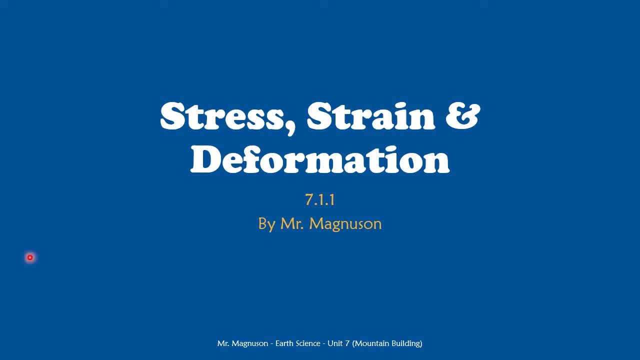 Welcome, ladies and gentlemen. Today we are starting a completely new unit. We are going to be talking about mountain building And, before we can learn about mountain building, we're going to do a little bit of rock engineering background work. today We are going to learn about the different ways that rocks can be changed or broken, And we're going 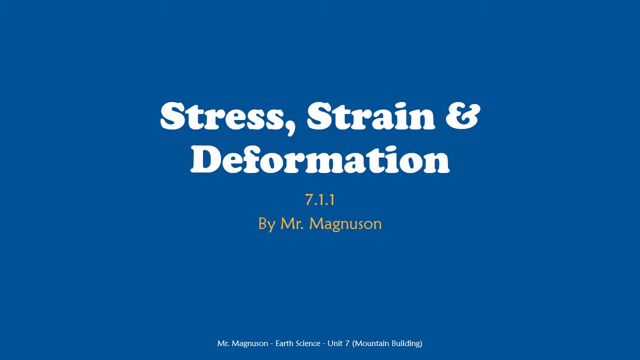 to be learning some general terms so that when we talk about processes that build mountains later on we will have some vocabulary to describe those terms. So let's jump right in. First off, what is stress? What is strain? We've got some words that we are going to be using. 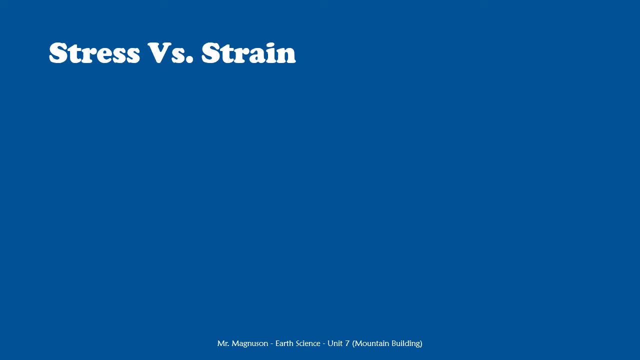 and you may not have heard them before. I want to make sure we're all on the same page, because we are going to be using words like stress, strain and deformation a lot in this unit to talk about processes that are happening to rocks. So when I talk about stress, 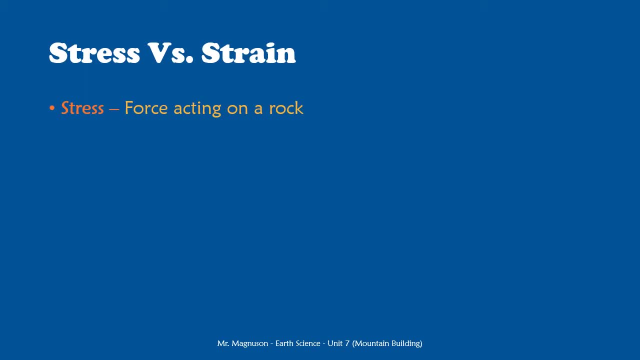 I am talking about a force that is acting on a rock, And we will a lot of times talk about the conditions under which that force is occurring. Is the force happening really quickly? Is it happening over a long period of time? Is it happening over a long period of time? Is it? 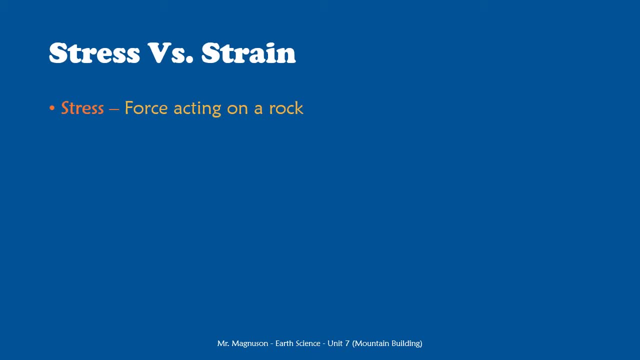 happening over a long period of time? Is it happening in a hot environment? Is it happening in a cold environment? These are the things we care about when we talk about stress. Next is deformation. So when a rock is deformed, it is changing shape, And when 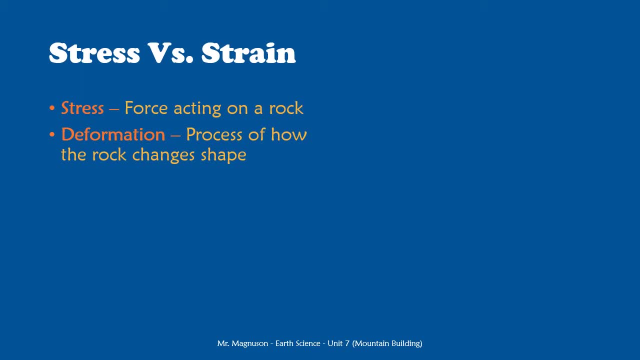 we talk about deformation. we are talking about the process of how that rock changes shape. Is it going to fold or bend or flow, Or is it going to like break or fracture? Those are kind of the big categories of deformation that we will talk about. 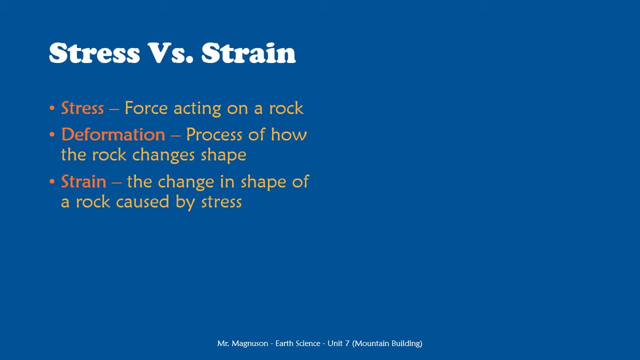 And finally, strain. Strain is the change in shape that is caused by stress. So the end result that we get after deformation happens is strain, And I want to show you a quick flow chart. The order that these things occur in is important, So let's look over on the 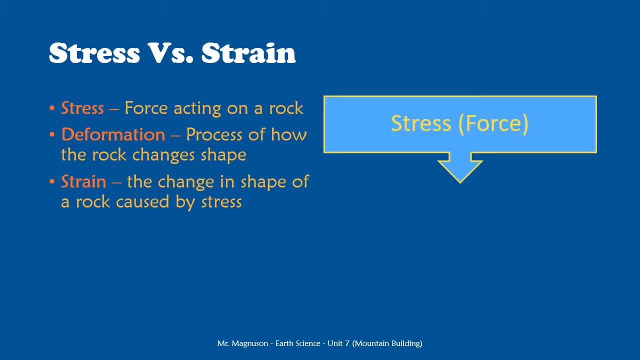 right-hand side. Stress is the force. Stress causes deformation, which is a type of changing of shape of the rock, And then, when you look at a rock after deformation, you can see that the rock is in a shape. And then, when you look at a rock after deformation, you can see that the rock is. 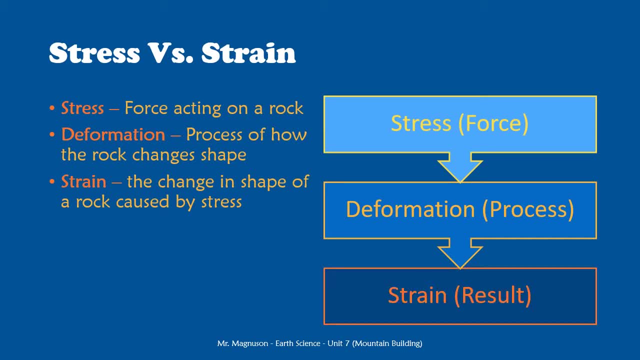 in a shape. And then when you look at a rock after deformation, you can see that the rock is in a shape. That result, that shape, you see whether it's a break or a fracture. that is what we call strain. Now, today we are going to be focusing on stress and deformation. different types of forces. 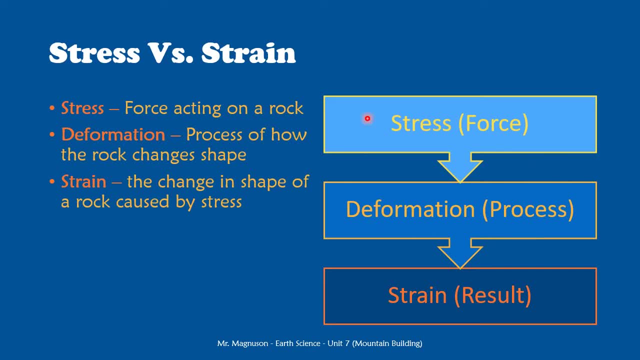 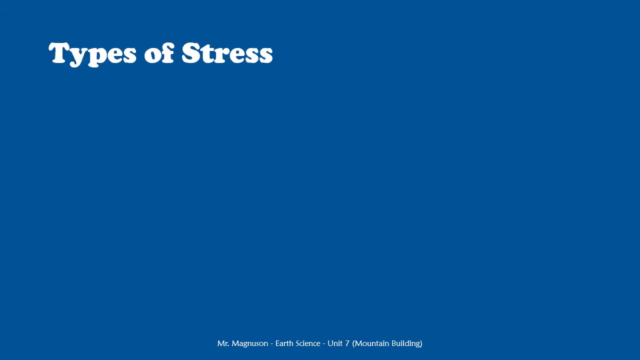 and the different processes of deformation, like breaking or folding, The different strains, the different features that we see formed by stress and deformation. we will be spending another lecture on those later. So let's look at types of stress. This is going to be pretty simple. The stress is the force that's acting on the rock. 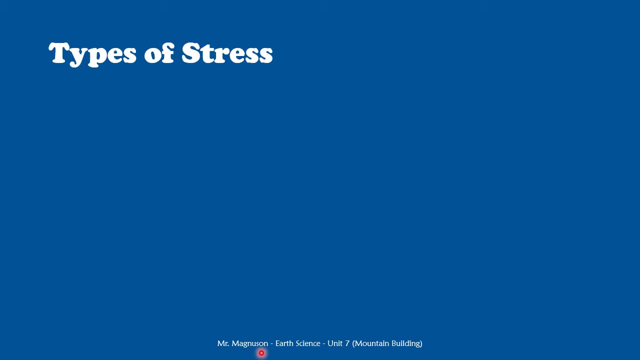 and here what we care about is the direction in which this force occurs, So we can have compressional stress. Compressional stress is when the rock is pushed together or shortened. You can imagine that this is going to happen very deep down in the earth, where pressure is causing. 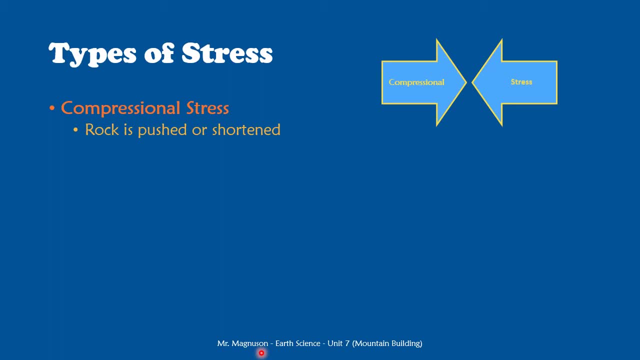 lots of compression, or you could imagine, maybe this is going to occur at convergent boundaries, where two plates are smashed, Excuse me. Next we have tensional stress. This is kind of the opposite of compressional stress. This is when rock is pulled or stretched, and you can imagine that this is going to happen. 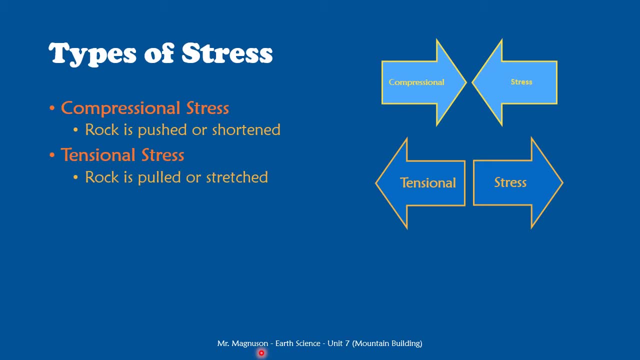 at divergent boundaries, at spreading centers, where we are pulling rock apart, And finally we have shear stress. Now shear stress is a little bit difficult to explain, because the important thing with shear stress is that the rock is either being stretched or shortened. 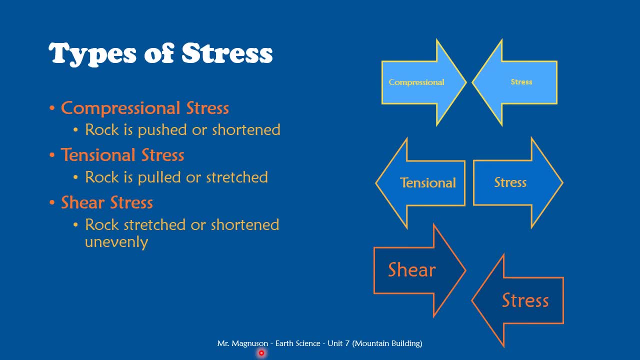 but it is happening in the earth, But it is happening unevenly. So you can see I've got my arrows over here lined up on the right-hand side, pushing- not right- against each other With shear stress. you can think of scissors. When you close scissors, they don't come together evenly. One blade goes on top of the. 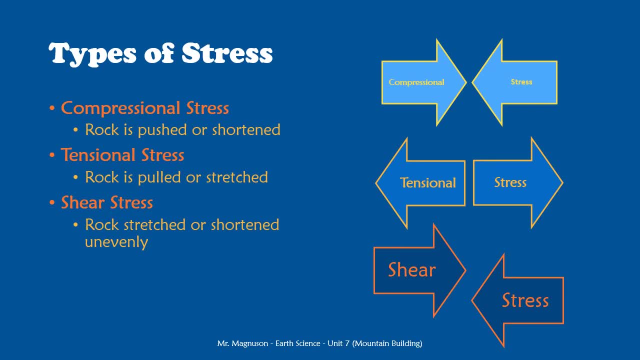 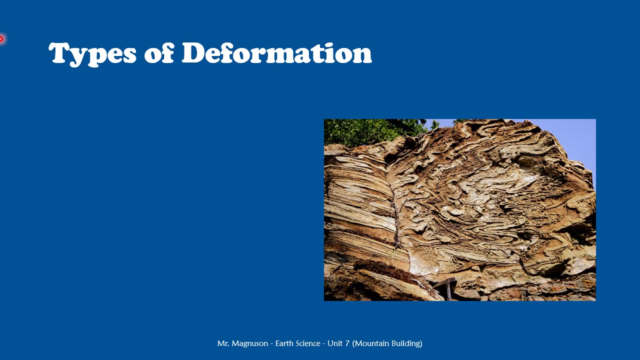 other, and so that is what we mean by shear. We are getting pressing or stretching, but it's happening unevenly. Next slide, Next slide. Let's look at our different types of rock deformation, The way that the rock changes shape. 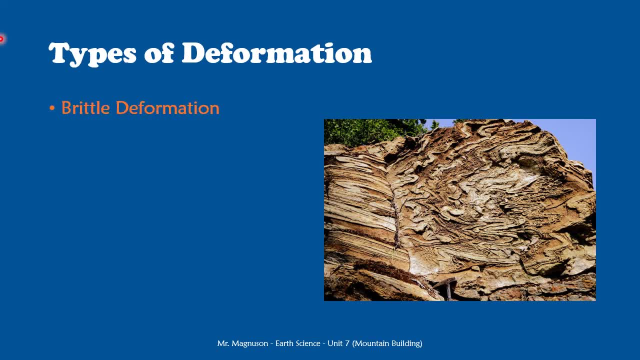 there's gonna be two broad categories that we learn about. The first is brittle deformation. Brittle deformation occurs when rock breaks into pieces in response to stress. These are things like breaks, faults, fractures, If you look closely at this picture right here. 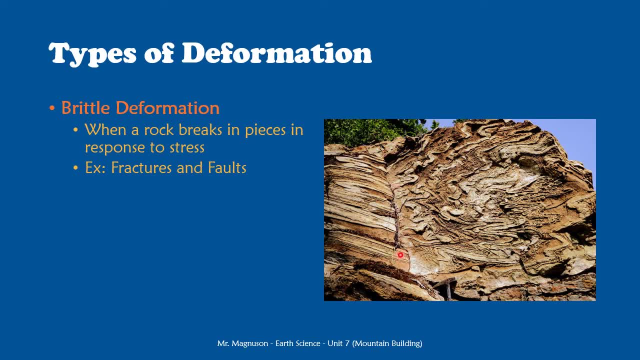 you can see this crack running along the left-hand side. This would be brittle deformation. Ductile deformation is our other type, our other way that rock can change shape. This is where we get bends or flows in response to stress, And you can see over here. 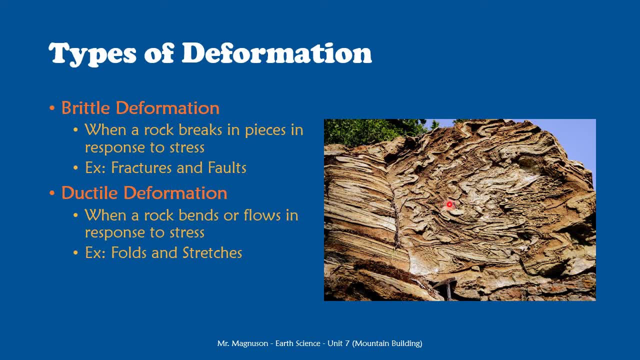 that on the right-hand side of this picture we have all these weird bends and squiggles in the rock layers. That would be an example of ductile deformation So important to remember: breaks equals brittle Cracks. breaks into pieces. Brittle folds equals ductile. 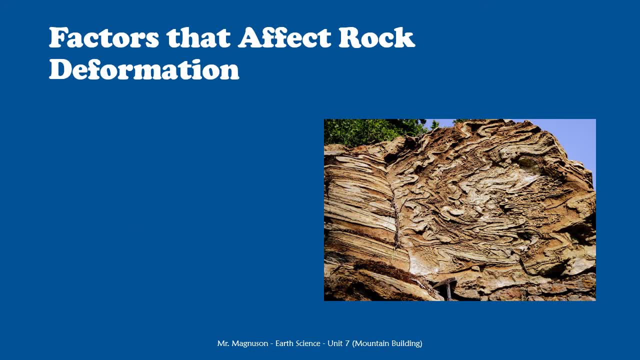 These are two types of deformation. The last thing I wanna look at today are factors that can affect rock deformation. So why are we more likely to see a break versus a fold? Why are we more likely to get brittle or ductile deformation? And again, remember: breaks equals brittle. 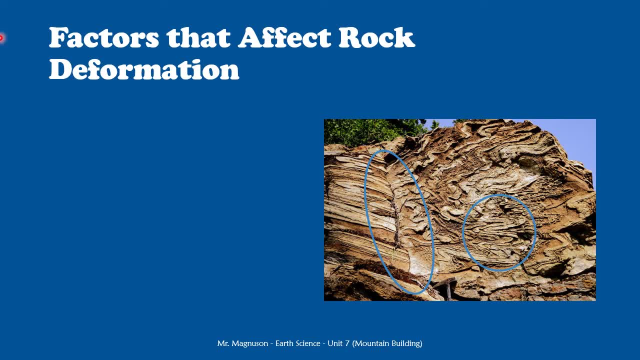 folds equals ductile, So we're gonna be looking at things that can affect how rock will deform form. These are going to be conditions under which our stress is applied. So first thing we're going to look at is temperature. We can have our stress occur at very low temperature. This is going to 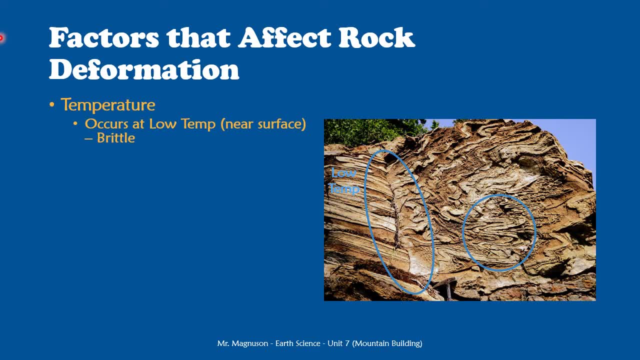 cause our brittle deformation. We can have stress occur at very high temperatures. This is going to cause our ductile deformation And you can imagine that low temperatures are going to occur near the surface. High temperatures are going to occur deep within the earth. That's how temperature 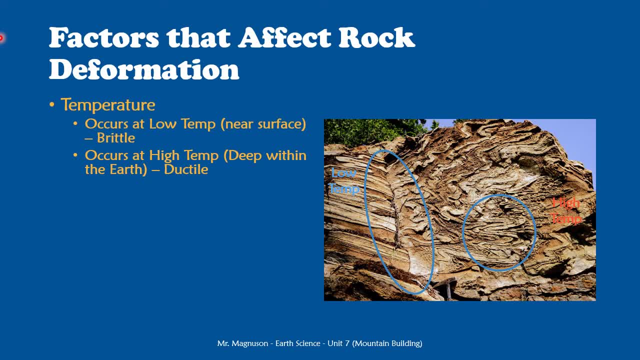 tends to change. If you want to think of these examples, think of me playing with that silly putty in class: The cold silly putty. if I tried to stretch it out it would snap very quickly, whereas the warm silly putty would stretch and form this really long, stringy shape.